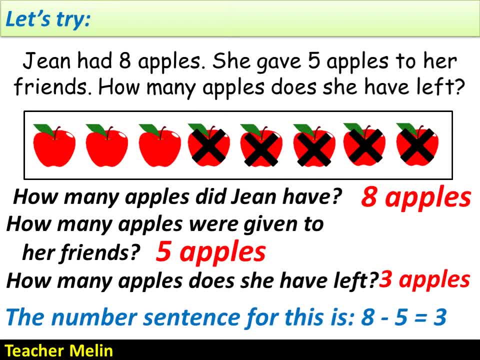 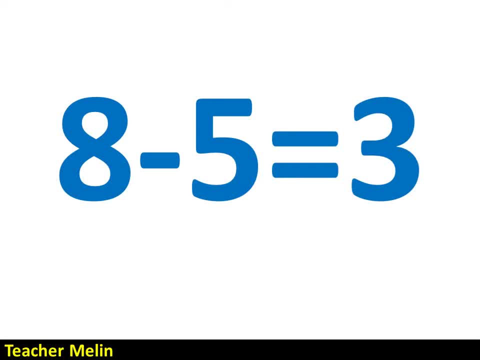 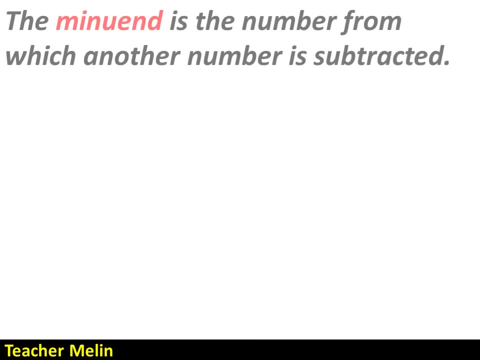 Eight minus five equals three. Eight minus five equals three. Eight is the minuend, Five is the subtrahend And this is the minus sign, And number three is the difference. The minuend is the number from which another number is subtracted. 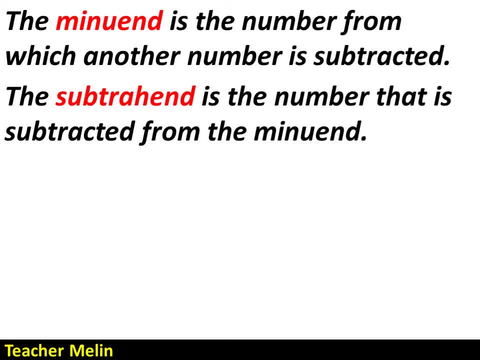 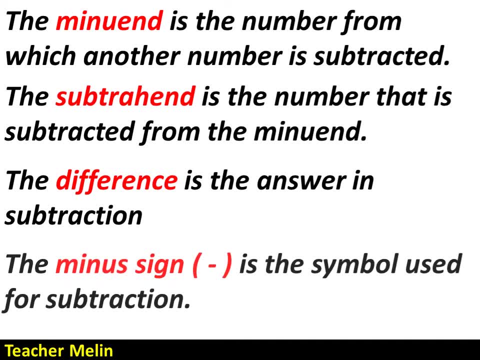 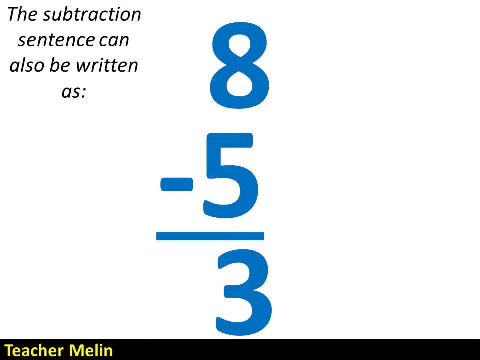 The subtrahend is the number that is subtracted from the minuend. The difference is: the number from which another number is subtracted is the answer in subtraction. the minus sign is the symbol used for subtraction. the subtraction sentence can also be written as: 8 minus 5 equals 3. 8 is the minuend. 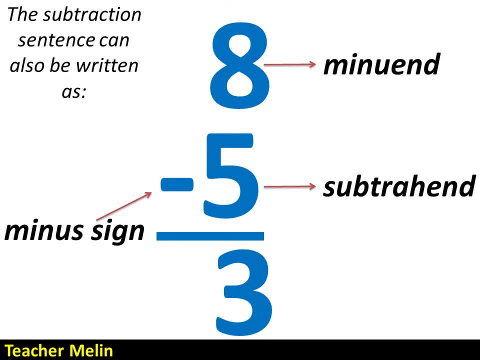 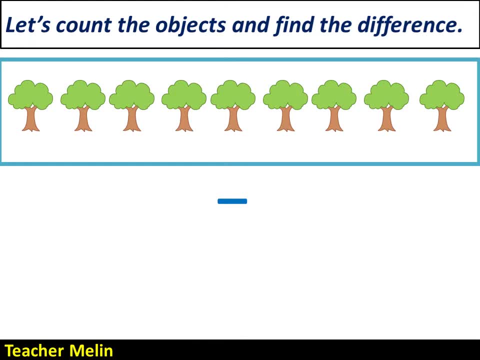 5 is the subtrahend and this is the minus sign, and number 3 is the difference. let's count the objects and find the difference. there are trees. let's count the trees ready: 1, 2, 3, 4, 5, 6, 7, 8. 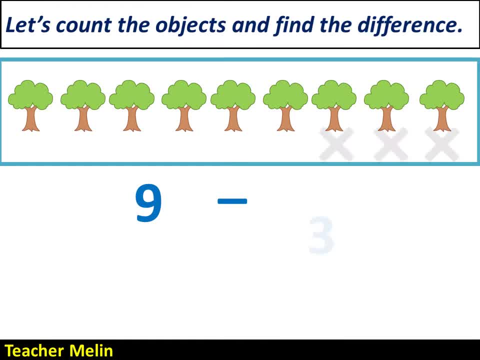 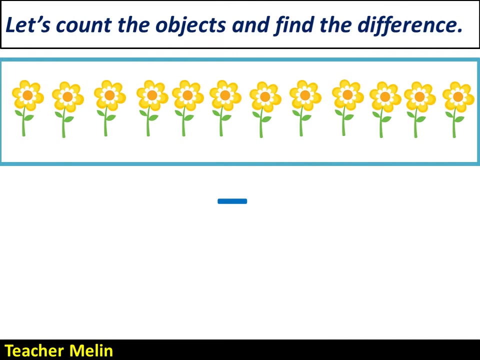 there are nine trees. let's take away three trees. how many trees are left? let's count 1, 2, 3, 4, 5, 6, 9 minus 3 equals 6.. another example: there are flowers. let's count the ready: 1, 2, 3, 4, 5, 6, 7, 8, 9, 10, 11, 12. there are 12 flowers. 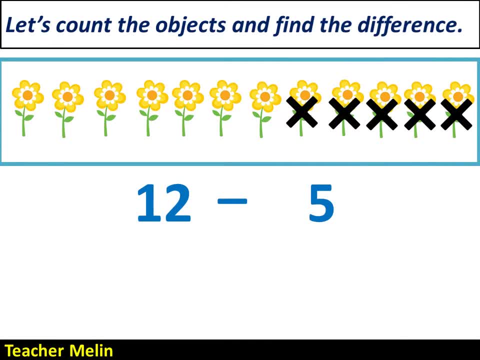 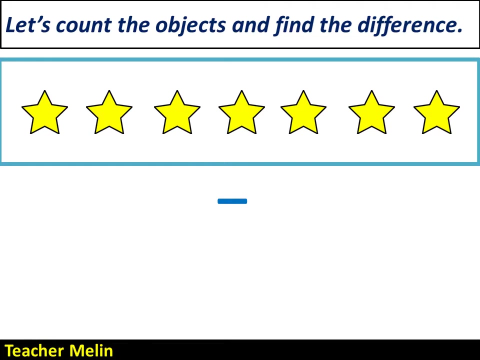 let's take away five flowers. how many flowers are left? let's count 1, 2, 3, 4, 5, 6, 9, 10, 11, 12, 5, 6, 7.. 12 minus 5 equals 7.. Another example: There are stars. Let's count all the stars. 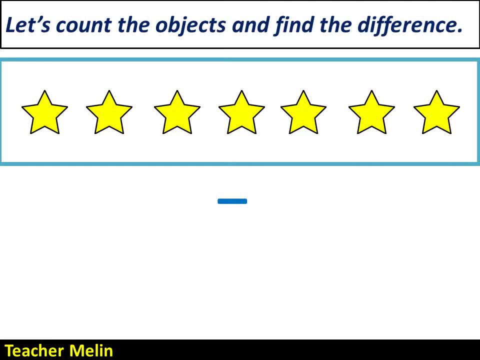 Ready: 1,, 2,, 3,, 4,, 5,, 6, 7.. There are 7 stars. Let's take away 2 stars. How many stars are left? Let's count 1,, 2,, 3,, 4, 5.. 7 minus 2 equals 5.. 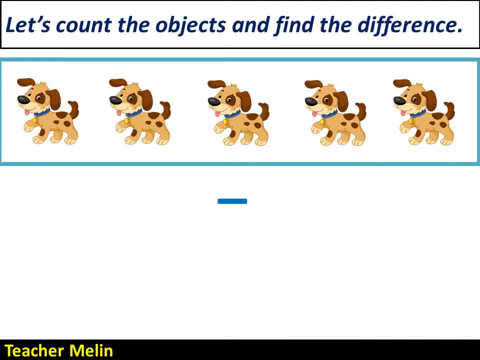 Another example: There are dogs. Let's count the dogs Ready: 1,, 2,, 3,, 4, 5.. There are 5 dogs. Let's take away 1 dog. How many dogs are left? Let's count. 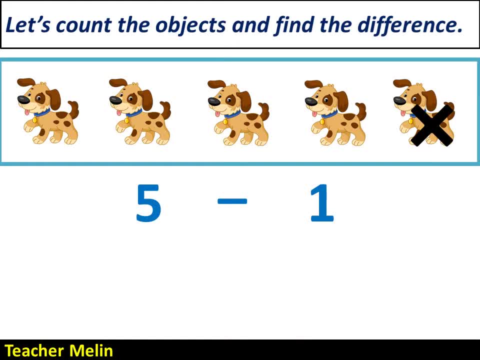 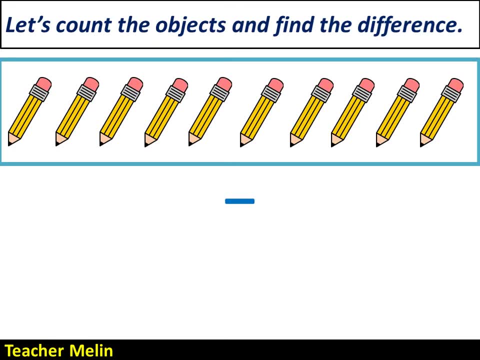 1, 2,, 3, 4.. 5 minus 1 equals 4.. Another example: There are pencils. Let's count all the pencils Ready: 1,, 2,, 3,, 4,, 5,, 6,, 7,, 8,, 9,, 10.. 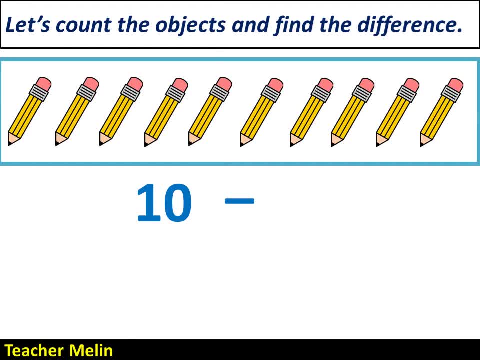 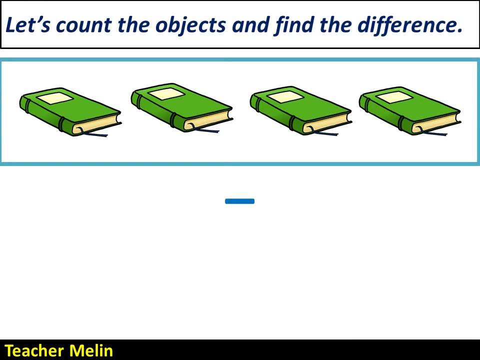 There are 10 pencils. Let's take away 6 pencils. How many pencils are left? Let's count 1,, 2,, 3, 4.. So 10 minus 6 equals 4.. Another example: There are books. Let's count all the books. 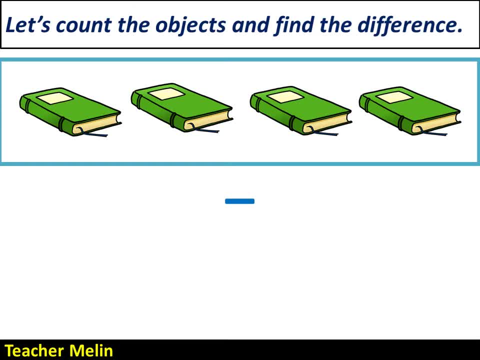 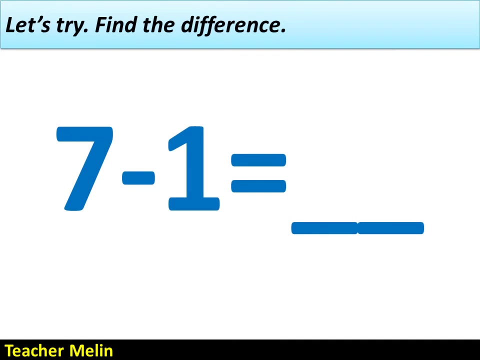 Ready: 1,, 2,, 3,, 4.. There are 4 books. Let's take away 4 books. How many books are left? 4 minus 4 equals 0.. Let's try Find the difference. 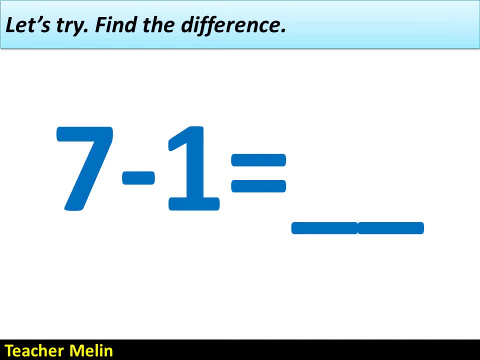 6. 7 minus 1 equals 6.. What is the correct answer? The answer is 6. 7 minus 1 equals 6.. Another number: 10 minus 3 equals 10.. What is the correct answer? 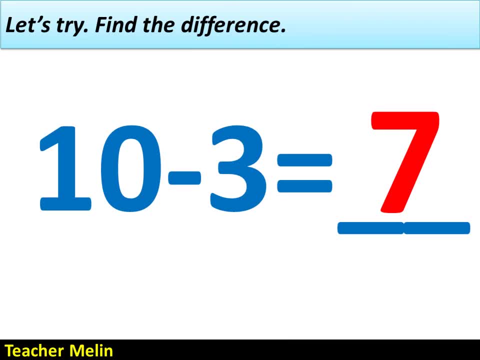 The answer is 5.. 7 minus 1 equals 7. 7.. 10 minus 3 equals 7. 5 minus 5 equals. What is the correct answer? The answer is 0.. 5 minus 5 equals 0.. 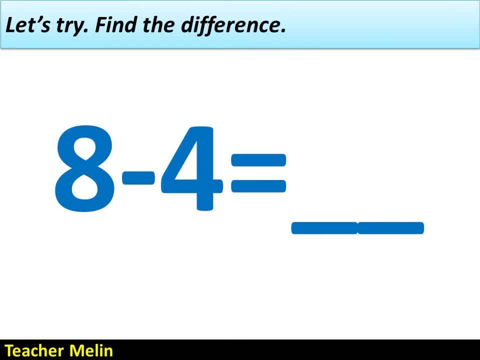 Another numbers: 8 minus 4 equals. What is the correct answer? The answer is 4.. 8 minus 4 equals 4.. 3 minus 2 equals. What is the correct answer? The answer is 1.. 3 minus 2 equals 1.. 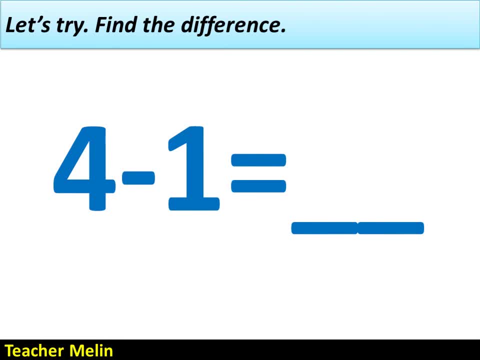 4 minus 1 equals. What is the correct answer? The answer is 3.. 4 minus 1 equals 3.. 9 minus 1 equals. What is the correct answer? The answer is 8.. 9 minus 1 equals 8.. 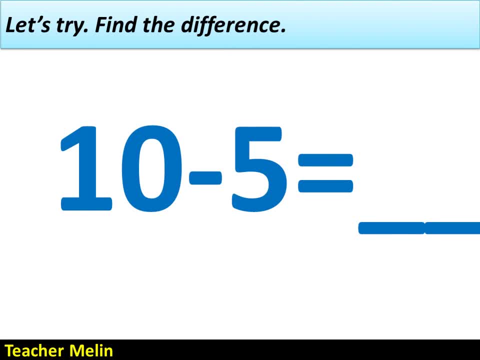 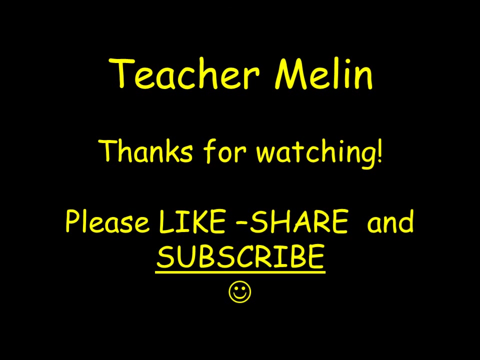 10 minus 5 equals. What is the correct answer? The answer is 5.. 10 minus 5 equals 5.. Thank you for watching.